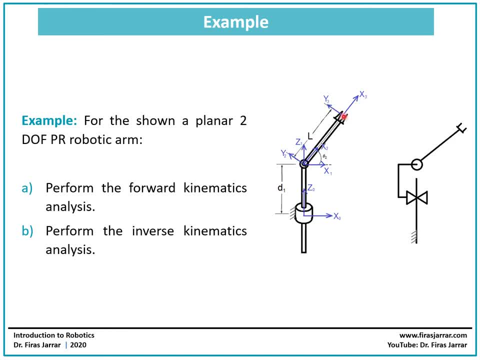 And Z three is out of the page for frame three, which is attached to the end effector. We have: D one is a variable joint for the prismatic joint and L is constant and theta two is another joint variable for joint two, And we are required to perform both the forward kinematics and the inverse kinematics for this simple two degrees of freedom. robotic arm. 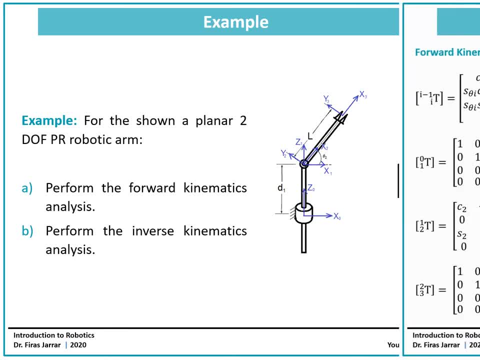 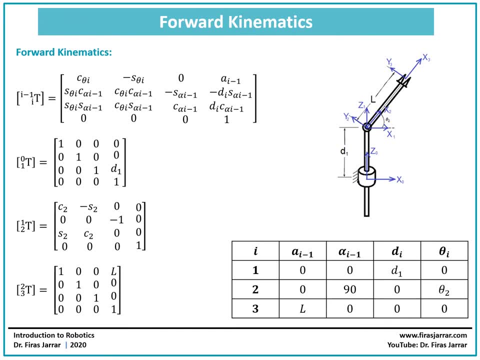 Here we're going to start with the forward kinematics. In the forward kinematics, first of all we need to determine the DH parameters. So, starting with the link, with the link length, a. so starting with a zero. a zero represents the distance along X zero between Z zero and Z one. 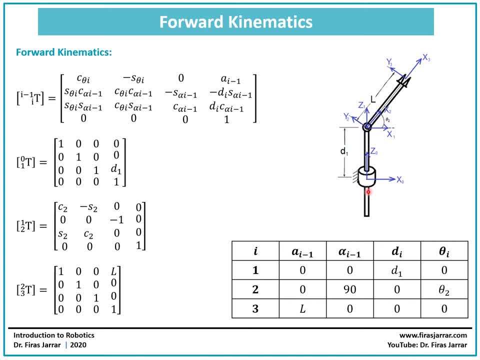 Z zero and Z one are coincident or parallel to each other along the same line. So X zero is going to be zero. Now for a one. a one is the perpendicular distance along X one between Z one and Z two. So this is Z one. here we agreed that Z two is out of the page. They both intersect at the same point along the X one direction. 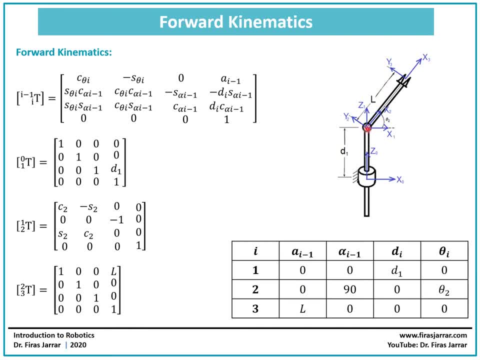 A two is the perpendicular distance along X two between Z two and Z three. So you can see that this perpendicular distance is equal to L. Then we're going to look at the link twist, starting with alpha zero. Alpha zero is the angle about the X zero between Z zero and Z one, And since both are parallel and they remain parallel. 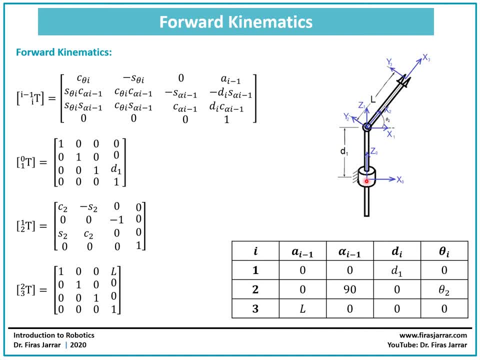 During the motion of the robotic arm. this is going to be a zero And then alpha four, alpha one And this is going to be the angle between Z one and Z two Along About X one. so Z one is upwards here to is out of the page. So the angle between Z one seconds to is going to be 90 degrees positive 90 degrees. 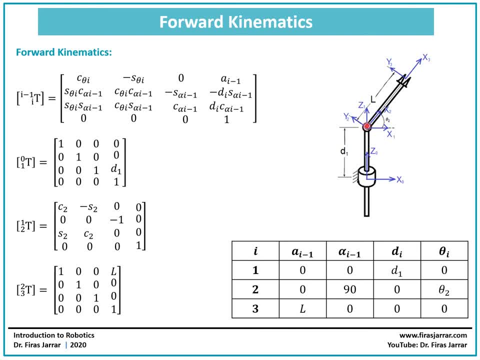 So, according to the right hand rule, you will have your. you need to have thumb pointing towards the x1. it's going to remain like that- pointing about x1. you have your fingers towards z1, your palm of your hand facing your, facing you, and then you need to rotate or curl. 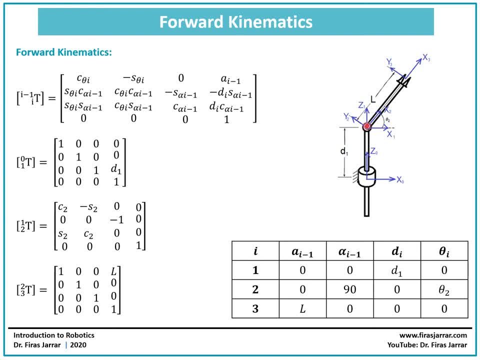 your fingers towards, from z1 towards z2, and this takes you at, takes you through an angle of 90 degrees. then, finally, we're going to look at alpha 2. alpha 2 is about x, it's about x2, between z2 and z3 and z2 and z3. both of them are pointing out of the page. they remain like that. so the angle. 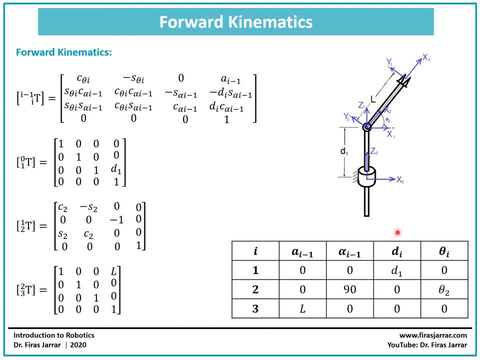 between them is going to be zero. now let's look at the link offset, starting with d1. d1 for d1 is going to be the distance along z1 between x0 and x1, the perpendicular distance between x0 and x1 along z1. so this is d1 here, which is a variable, d2 is the perpendicular. 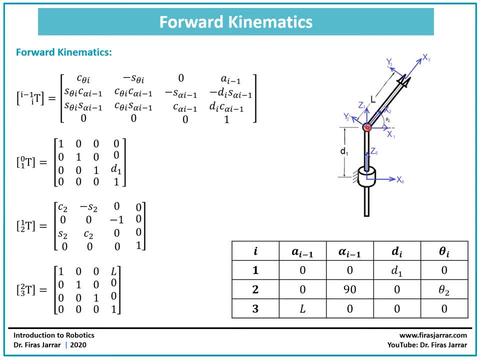 distance along z2 between x1 and x2. they are both intersecting at the same point along z2, so this is going to be z1 and x2 here. and for d2 is the perpendicular distance along z3 between x2 and x3, and this is going to. 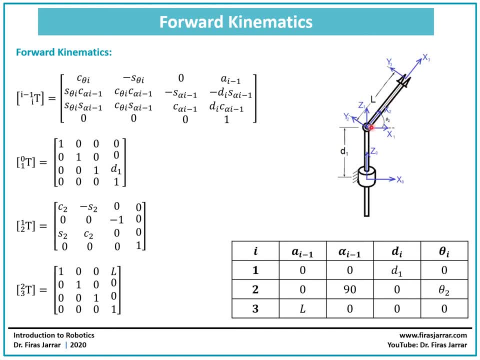 be equal to zero, because they are both collinear and parallel, intersect along at the same point, along the z3, so this is going to be zero here. then, finally, we have the joint angles, we have theta one. theta one is the angle about z1 between x0 and x1, and this angle is about z1 between x0 and x1, and this is going to 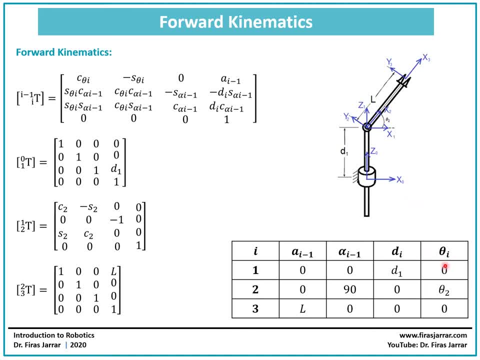 be constant because they remain parallel to each other, and it's going to be equal to zero. theta 2 is the angle about z2, between x1 and x2, and this is variable and it's going to be equal to theta 2. and finally we have the. theta 3 is an angle about 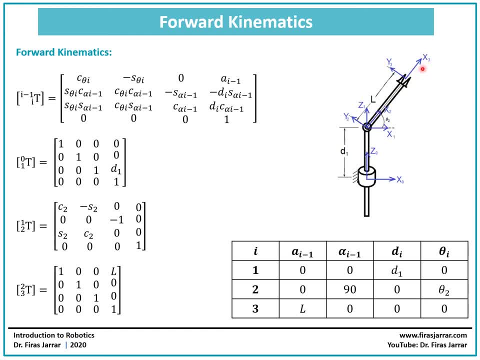 z3 between x2 and x3. x3- and these two are parallel- will remain parallel and thus it's going to be equal to zero. so these are the dh parameters for this robotic arm. the next step in the forward kinematics is to substitute for the each. 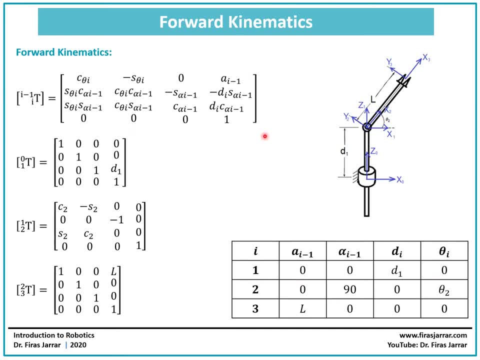 each row into the general homogeneous transform matrix for each link. so starting with i1, and then we'll have t1 with respect to 0, the transformation matrix of frame 1 with respect to frame 0, and you need to substitute these values for theta d, alpha and a. 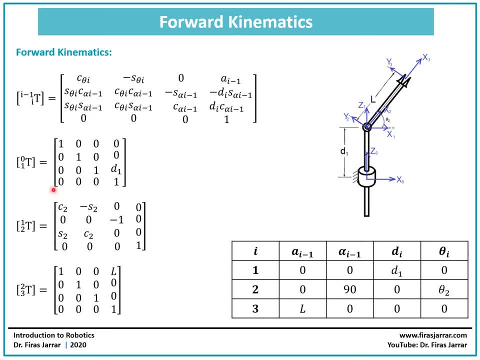 into this matrix. if you do this, you're gonna obtain this result here for t1 to 0. if you do it for the second row, this is the matrix that you will get, and if you do this for the third row, this is the matrix that you're going to obtain. now it's it's recommended always to double check. 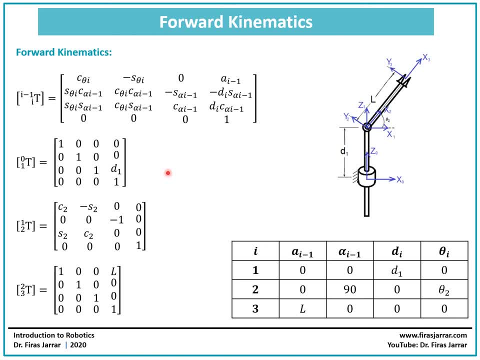 your answers and see if they make sense or not. so if i look at the transformation matrix for t 1 to 0, you can see that frame 1 compare frame 1 to frame 0, you can see that they are parallel and they will remain parallel because this is a prismatic joint allowing only for linear motion. so 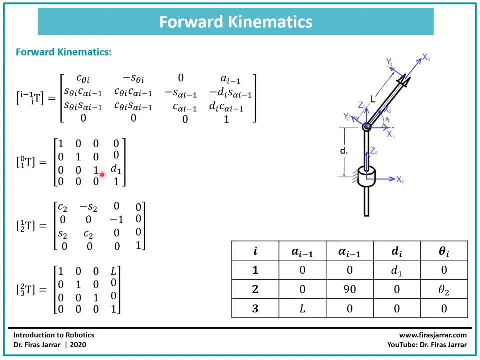 this part. here will be the identity matrix, which makes sense. then look at the origin of frame 1. origin frame 1 is translated along the z-axis, along z0, by distance of d1. so we'll have 0, 0 d1 here. this corresponds to the x coordinate, y coordinate and z coordinate. so it makes sense. 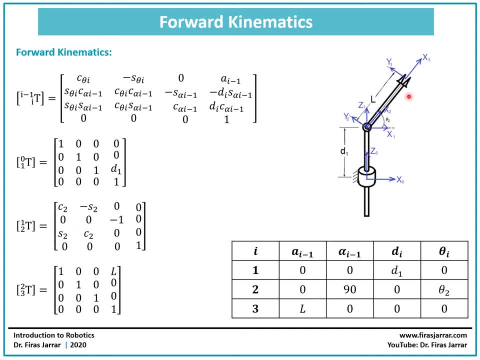 this one. and let's look at t 2 to 1. t 2 to 1 represents the t1 to 1 and t2 to 1 represents the orientation and position of frame 2 with respect to frame 1.. you can see we have x, y here, but we 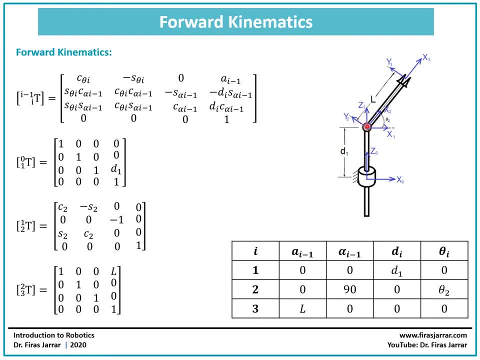 have x and z here, so we have not one basic rotation but rather two basic rotations. so it will be difficult to judge this one just by inspection, but at least we can say that this is correct. the position of the origin of frame 2 with respect to frame 1. 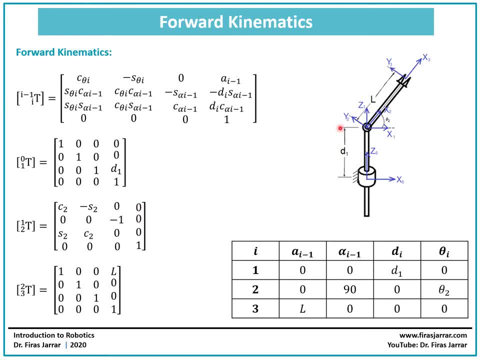 is at 0 0 0 0, because they have the same origin here. and finally, frame 3. with respect to frame 2, they'll remain parallel and this is why we have the identity matrix here and you can tell that frame 3 is translated along the x-axis x2, as we can see here, along x2. 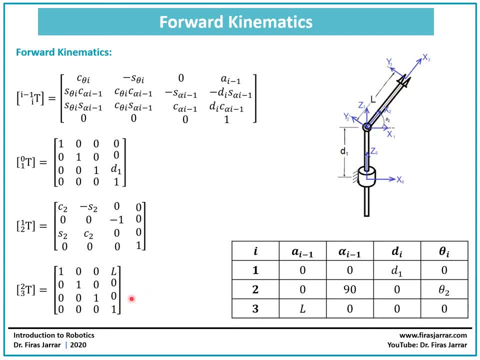 by a distance of l, and so this also makes sense and it's always going to be the same. and then the next step of your problem will be to multiply the transformation matrix at the end of the frame 2. here we show at the Carmen. if the end is basically equal to the 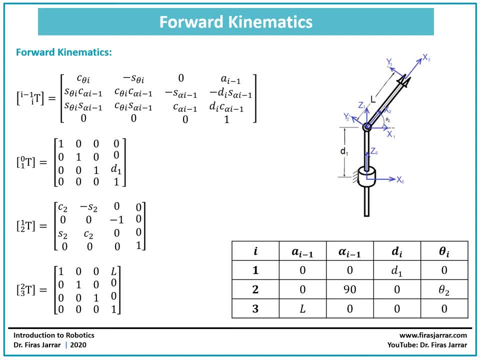 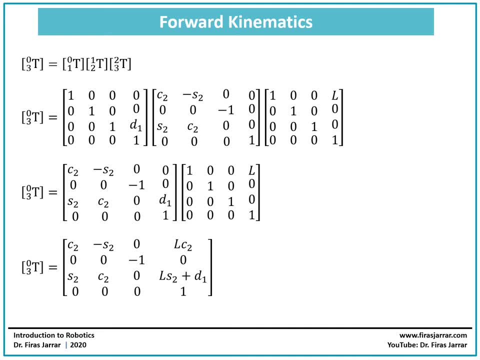 frame one. we're going to have x at the side with respect to this transformation matrix. so we're going to. why do we need to multiply this transformation matrix to find proof? what's the Bonetti proof? so one notice: if the 21 x22 24あ. 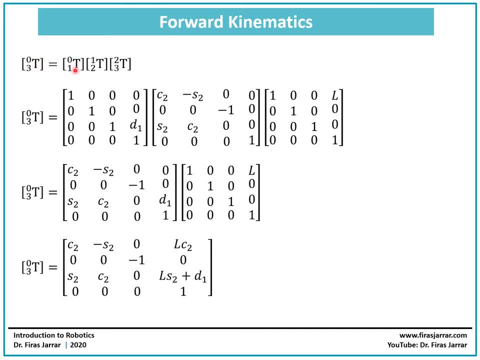 with respect to frame 0, i need to multiply t 1 to 0 by t 2 to 1 and t 3 to 2, and we- this is going to be a simple, especially in this case, where we have identity matrices hidden here- and this would be the final result. so you start by multiplying, multiplying this matrix. 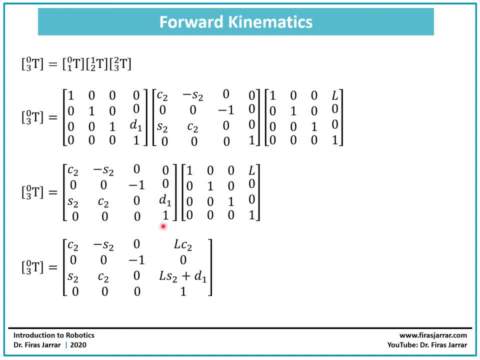 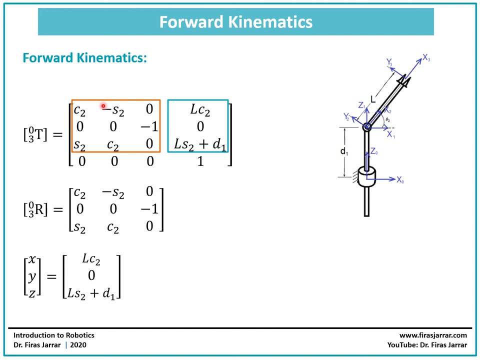 by this one, and this could. this would be the result here, and then you multiply this matrix by this one here to get the final result of the forward kinematics. so this is a summary of the results that we got for the forward kinematics. this is the transformation matrix representing the orientation and position of the end effector. 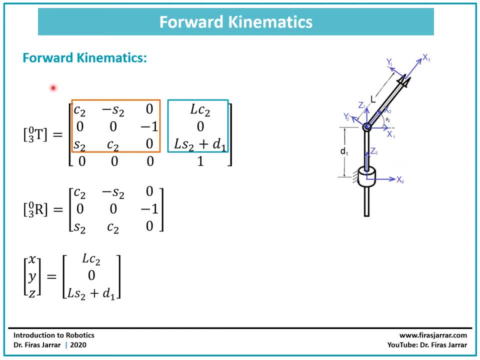 frame. frame three: with respect to frame zero, the transformation matrix consists of two sub matrices. one would be the rotation matrix here, which is r3 to 0, which represents the orientation of this frame with respect to the base frame, and this here in blue represents the position of the origin of the end effector with respect to the base frame. 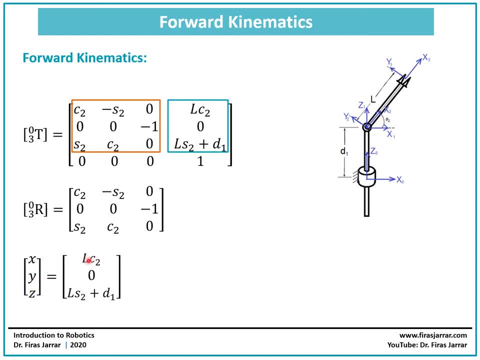 so we have x, y and z here, x being l cosine theta 2, y being always equal to 0 and z being equal to l sin theta 2 plus d, 1, and this is the orientation here. so, just as a reminder, the the result of the fourth kinematics. it simply gives us the orientation and position. 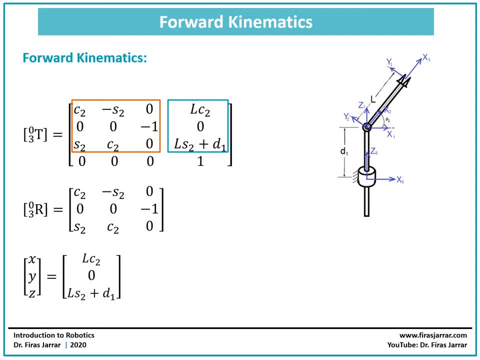 of the end effector frame with respect to the base frame. so you are simply answering the question: where is my hand, or where is the hand of the end or the end effector of the robotic arm? and for us, for human beings, be a silly question: where is my hand? and because we, honestly, we don't think about this. it's done. 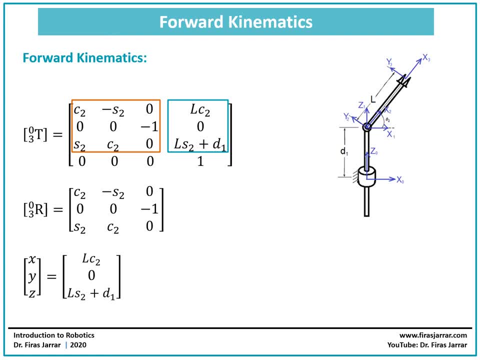 by the, automatically in the subconscious, and you don't need to worry about really figuring out where is your hand before reaching out to grab another object or a certain object. where it comes to robotic arms, no, this is becomes an important task and you need to really program it within. 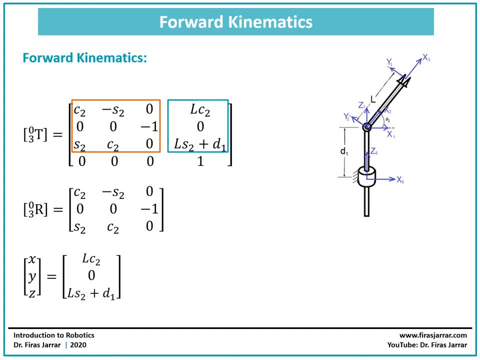 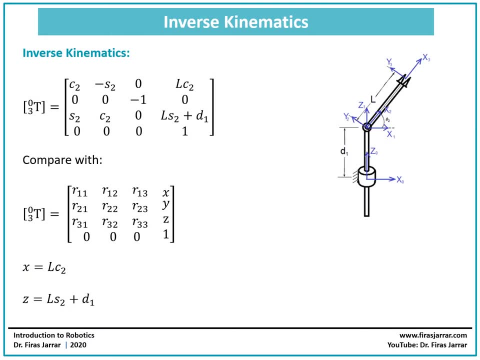 your robotic arm. now we'll proceed with the inverse kinematics. so this is the transformation matrix as we obtained from the forward kinematics and this is the general transformation matrix for an end-effector with respect to the base frame. we have general values. here could be any values. 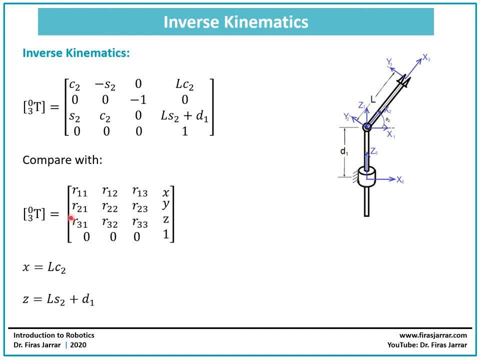 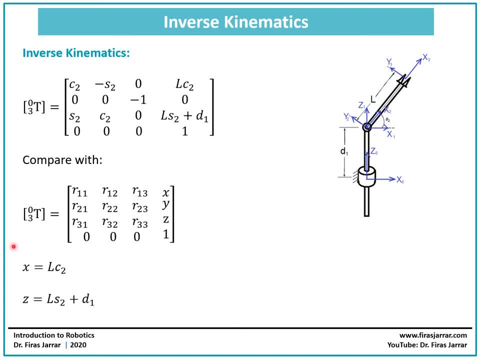 always part of the inverse kinematics. you want to simplify things. write it in the most general case, which applies for any robotic arm. compare it to the one we obtained from forward kinematics and you will see that it is always going to be 0.. that X is going to be L cosine theta 2 and the Z, in this case, is going to be L sine theta 2 plus d X. 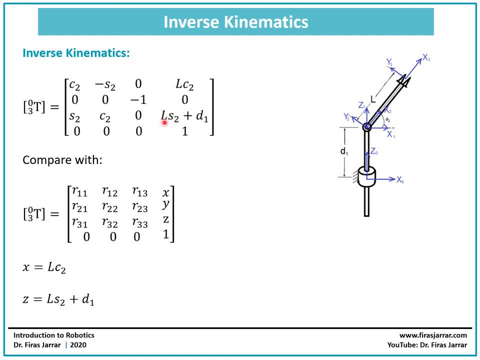 here and here we have the Z. now the goal is to from this problem. you need to figure out what are the values for theta 2 and the value for day D 1, in order to accomplish a certain X and Z, and values for the end effector. so the inverse kinematics is the opposite of the four kinematics. 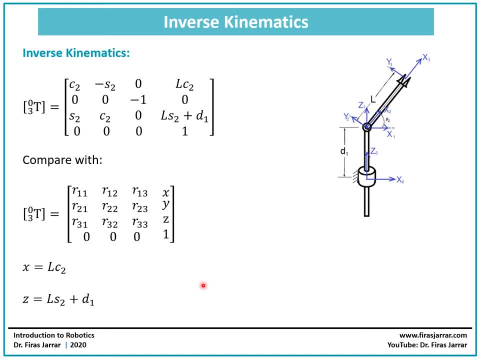 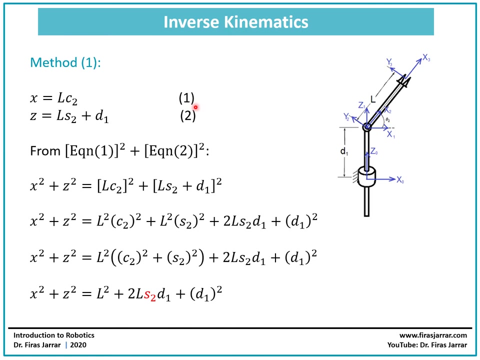 problem. now you have a certain value, a desired value or or a position for the end effector, and you need to determine on the joint variables which will take you there, the d1 and theta2 in this case. starting with these two equations that we obtained in the previous slide, an equation for X an. 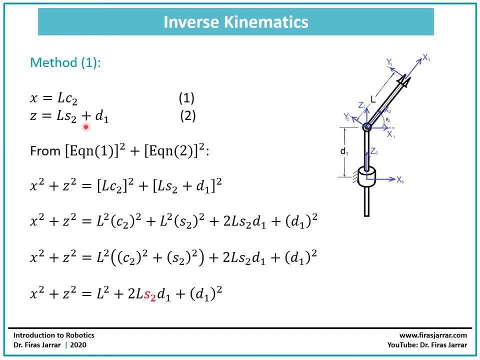 equation for Z. again, the goal is to to explicitly find a relationship or expression for theta2 and another one for d1. we're gonna use two methods to solve our inverse kinematics in this lecture. in the first method I'm going to start with the inverse kinematics and the first method I'm going 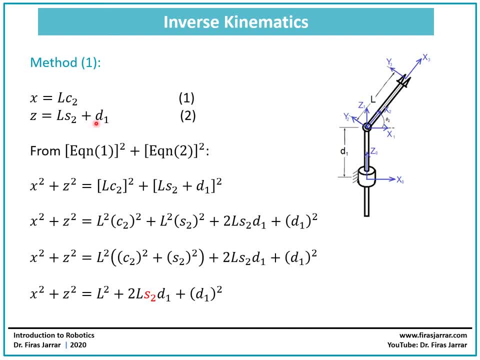 to start with the inverse kinematics and the first method. I'm going to start with the inverse kinematics and the first method. I'm going to start by looking at d1. I want to find a value for d1 as a function of X and Z and L, with no dependence on theta2 to do this. I'm gonna try to. 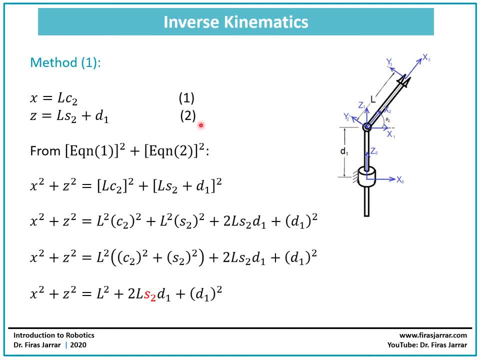 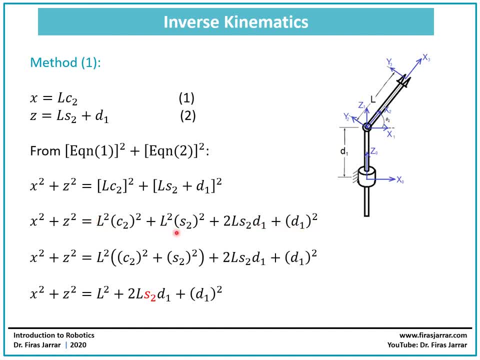 now you group these two terms together and you're going to notice that here we have a trigonometric identity which says that cosine theta 2 squared plus sine theta 2 squared is going to be equal to 1. so, and this will bring us to: x squared plus z squared is equal to l squared plus 2l sine theta. 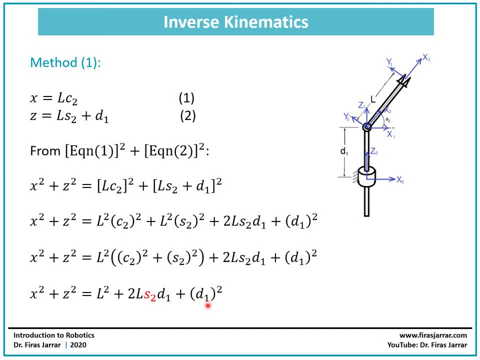 2, d1 plus d1 squared. however, we didn't reach our goal. you can see that we still have both d1 and sine theta 2, so we have two- these the two joint variables, theta 2 and d1, in the same equation, and the idea is to try to have only one joint variable first. so we'll, and our goal was to only. 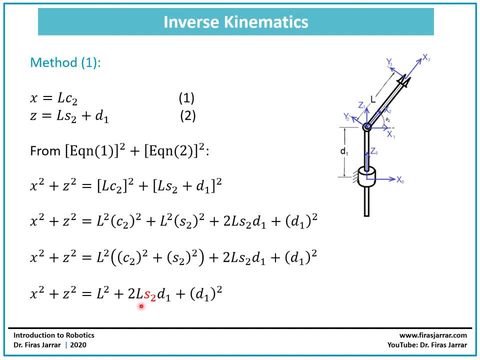 have d1 or only in this equation. remember that x and z and l are all joint variables, constants in the inverse kinematics problem. x and z are the coordinates of desired point for the end effector and l is a physical dimension, is the length of link 2. so how to proceed? we're. 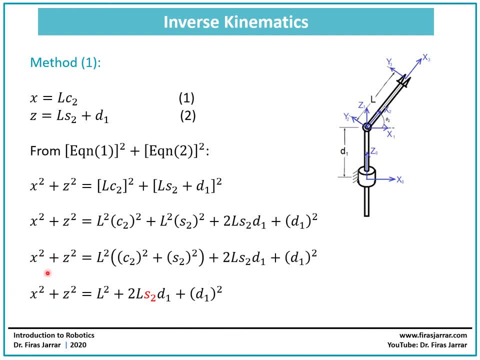 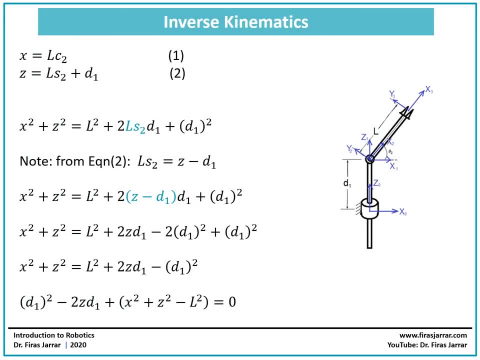 going to take this equation to the next slide and we can notice that l sine theta 2 appears in the second equation. so then it's possible to rewrite the second equation as l sine theta 2 is equal to z minus d1 and substitute the value for l sine theta 2 into. 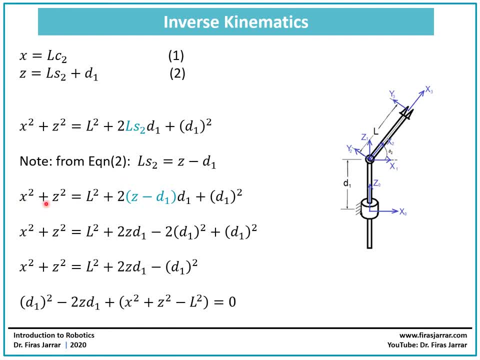 this equation. so now we'll have: x squared plus z squared is equal to l squared plus 2 times z minus d1, all of this times d1 plus d1 squared. so now we have x squared plus z squared squared. this way you can see that we eliminated theta 2 from the equation, and this was our goal. 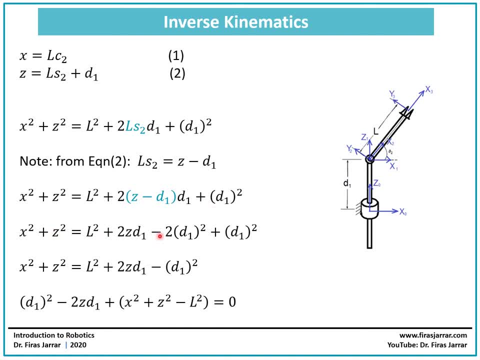 from the beginning. now, after a little bit of manipulation, you will have 2 z d1 minus 2 d1 squared plus d1 squared. so it becomes minus d1 squared here, and i want to rearrange the equation such that i have d1 squared minus 2 z d1 plus. 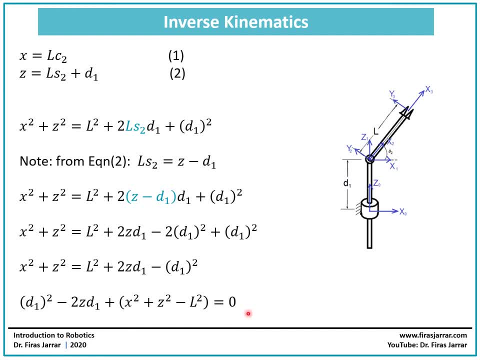 x squared plus z squared, minus l, 1 squared, all of this is equal to 0.. it looks like a quadratic equation because it is a quadratic equation. just keep in mind that it looks a little bit different than what we used to see in other courses, because in other courses, 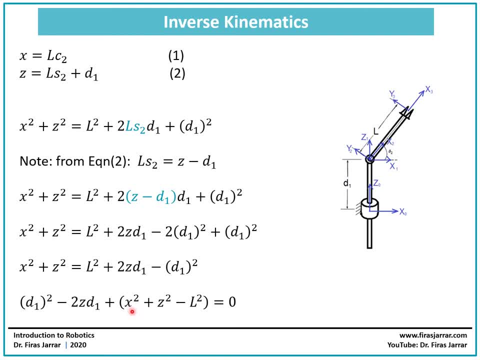 usually the x is the variable or the z is a variable, but here z and x are known, known values. so this is x squared plus z squared minus l squared. all of this is a quadratic equation. like a constant here and the d here is a variable. z is a constant and the d is also a variable here. 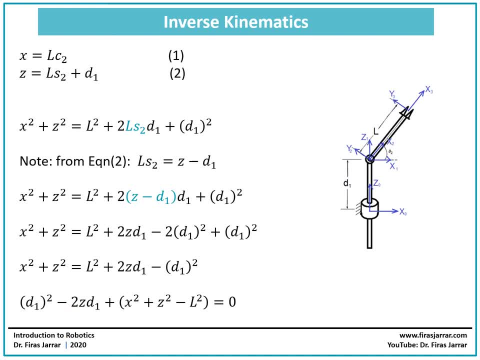 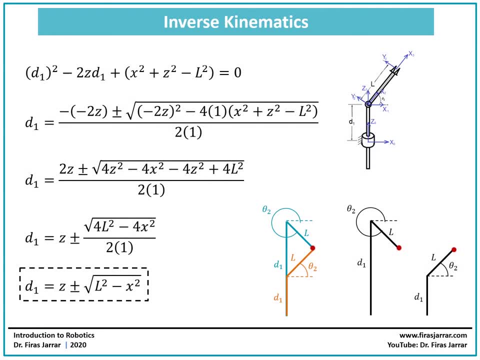 so this is a quadratic equation where we want to solve for d1. now we can use the general quadratic equation formula, for which we have d1 here and then we have minus. usually we call this b. so minus d, minus 2z and plus minus. under the square root we have b squared minus 4a. a is here one? it's going to be the one. 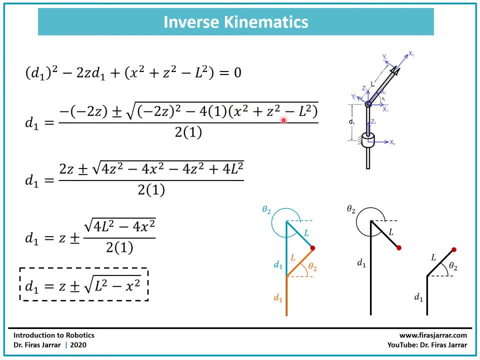 and multiply by c, which is s squared plus z squared minus l squared. all of this divided by 2 times a, the coefficient of the variable. here- this is a quadratic equation- can be simplified: the minus sign will cancel out. 2 will cancel out with the 2 here, so we'll have a z. 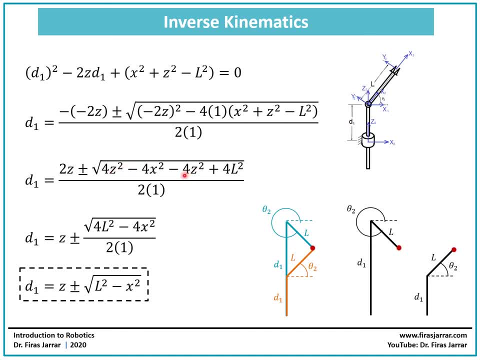 4z squared will cancel out with the minus 4z squared and the 4 can be taken out of the square root to become 2 and cancel out with the 2 here. so we'll have: d1 is equal to z plus minus the under square root l squared minus x squared. 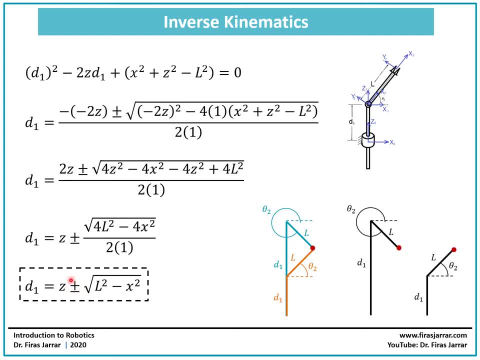 so the interesting thing here, that is that we have two solutions, one plus and one negative, and here i have in the figure a representation of the robotic arm. here we have the length d1, which is the joint variable, the prismatic joint variable, and i have l this 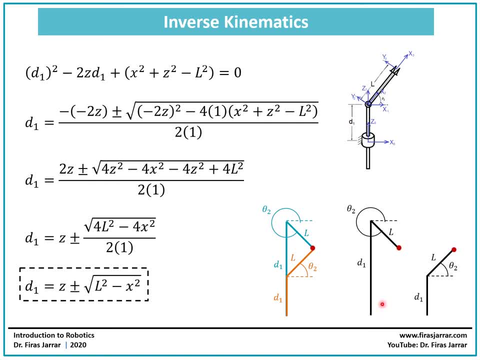 corresponds to one solution. and here i have another solution where i have d and i have l. both of them will give me the same end effector position. so the red dot here represents the end effector, end effector, the difference between. so this is solution one, this is solution two. 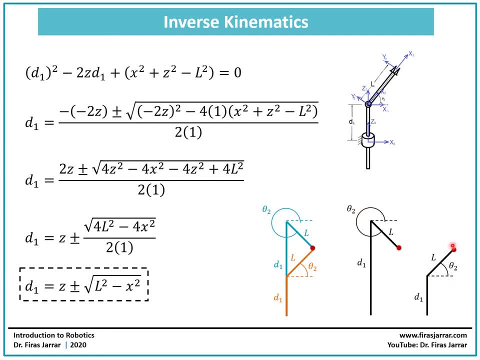 the difference between both solution is that here the robotic arm is pointing upwards, here the robotic arm is pointing downwards, both of them pointing towards the same end: effector point. I have superimposed both solutions on the same figure here, The first one, the first solution, being in orange. 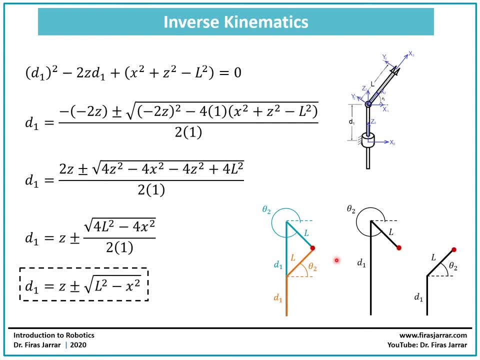 The second one being in blue color, So you can see they would reach the same position. So this really verifies our solution here That there will be two solutions for D1, And you can see that it depends on Z, L and X, Which are all given values. 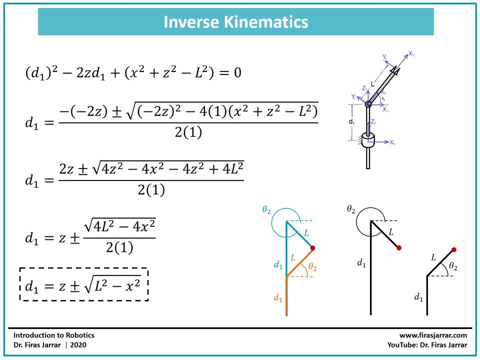 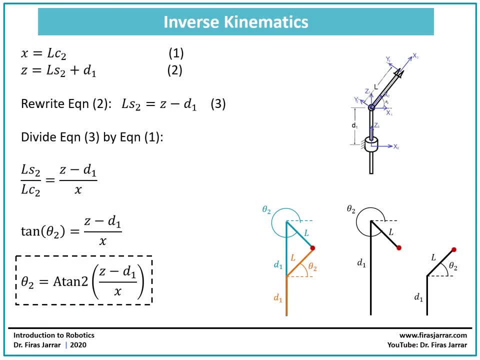 Now we need to proceed for theta2. So if we have D1, The problem of finding theta2 becomes much more easier. The second equation can be written as: L sine theta2 equals Z minus D1. D1 is known value now Has a known value. And if you take equation 3 divided by equation 1, 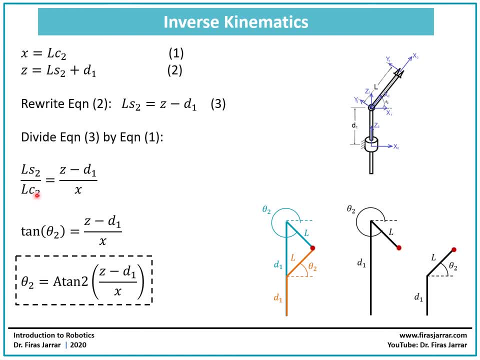 We will have L sine theta2 over L cosine, theta2 Equal to Z minus D1 over X, And L will cancel out with the L Sine over cosine. this is a tan Tan. theta2 is equal to Z minus D1 over X, And thus we can find theta2 as the tan inverse of. 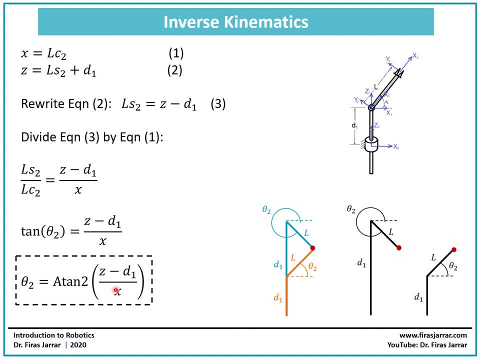 Z. Z is known, X is known And D was found in the previous slide, And you can see that theta2 depends on D1. So this is the first solution. for D1, There will be a corresponding theta2, Which is, in this case, in the first quadrant. 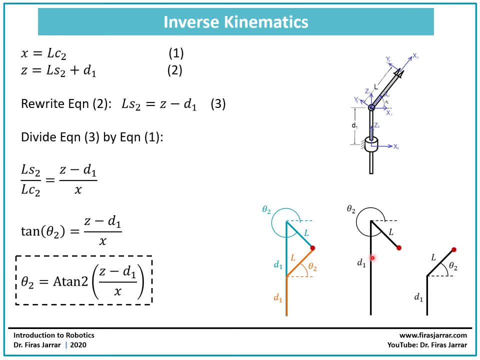 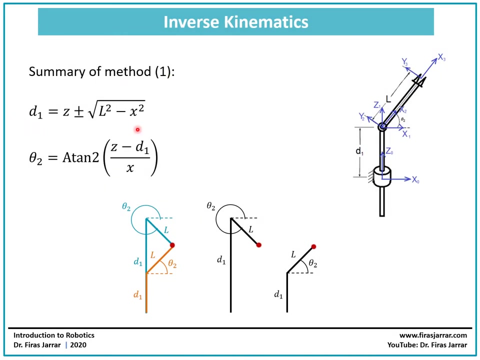 And for this larger D1, Representing the second solution, We will have another value for theta2 Which, in this case, is going to be in the fourth quadrant. Summary of method 1. We will have two formulas, two equations, One for finding D1 and one for finding theta2. 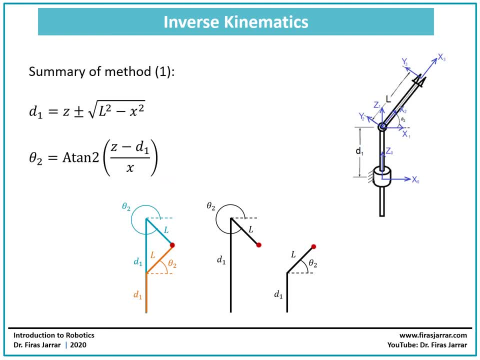 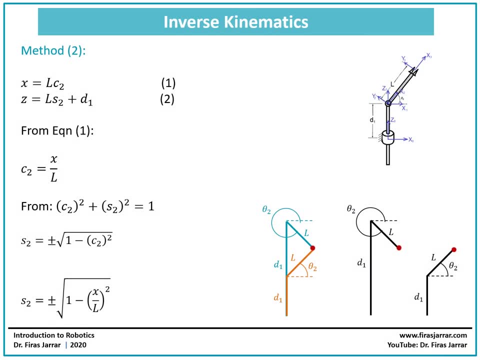 In the next slide we are going to start with method 2 In method 2, now we are going to start looking for theta2. In method 1, we started by first looking for a value for D1, But now we are going to start by looking for a value for theta2. 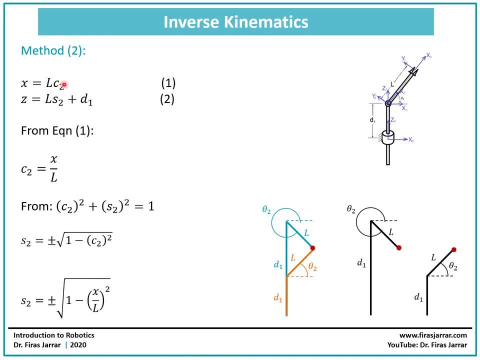 Now you can see directly from equation 1 We can obtain cosine theta2, Which is X over L, And from the general trigonometric identity, Which is cosine theta2 over L, sine theta2, Because cosine theta2 is equal to one, We can find that sine theta2 is plus or minus. 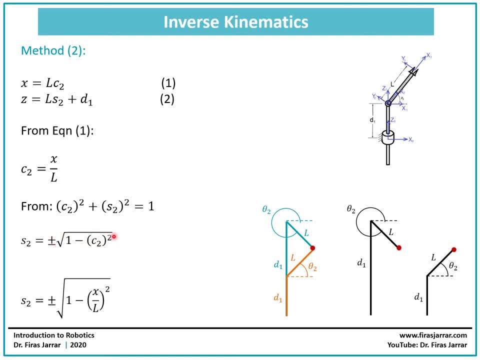 Under the square root, one minus cosine theta2 squared. If you wish, you can substitute for cosine theta2 here To have it as X over L, And now we have a formula for sine theta2 And we have a formula for cosine theta2. Now what you will see is that theta2, which is theta3, and theta4 is a sine theta2. 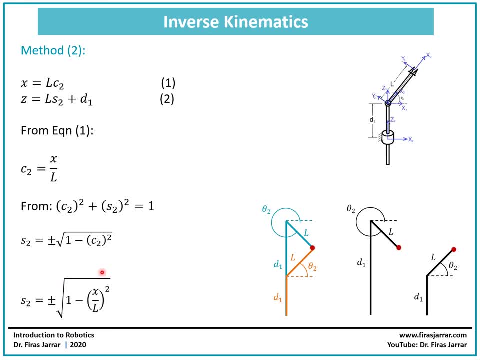 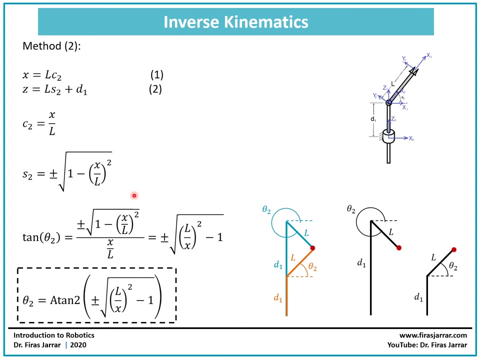 we'll have. obviously we're going to have two possible solutions, and this makes sense also from our previous presentation. theta 2 could be, for example, in the first quadrant or in the fourth quadrant. so once we have cosine theta 2, we have sine theta 2 dividing sine by the cosine we're. 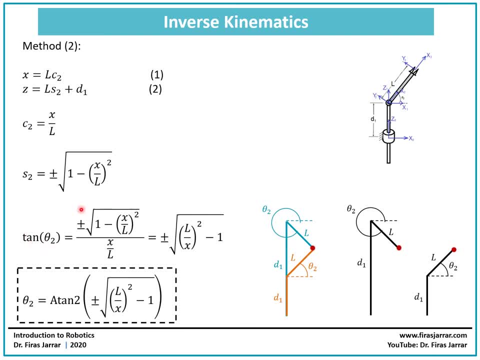 going to get a formula for tan theta 2 and if you wish, you can simplify these things by getting the x over l into inside the square root here and you will obtain a formula for theta 2. so theta 2 is going to be a tan 2 plus minus, representing two solutions in one solution. we can consider the plus. 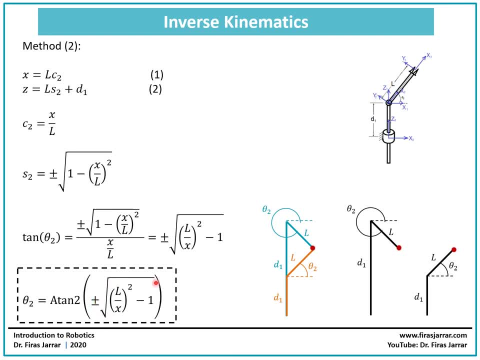 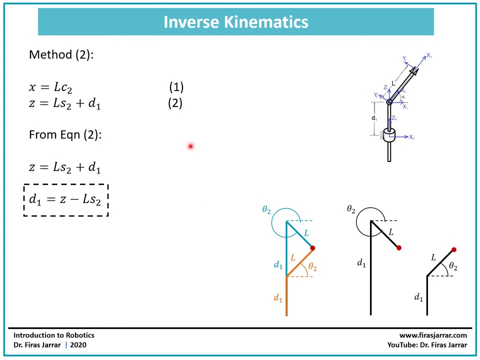 and the other solution, we can consider the minus and that the square root will have l over x squared, all of this squared minus one. after obtaining a value for theta 2, we can now proceed for looking, looking for a value for d1, and we can obtain this from equation 2, which is the only equation that has d1 in it. so we will 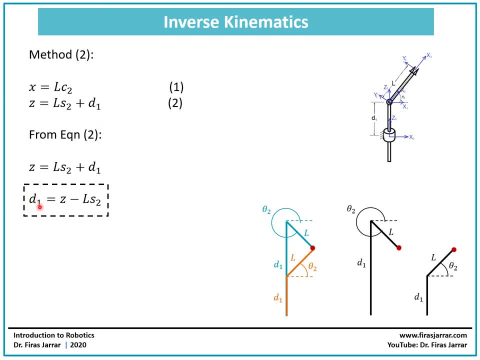 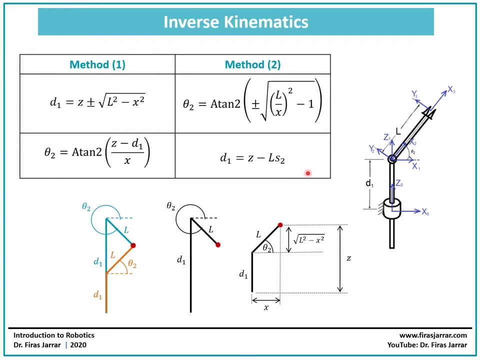 rearrange equation 2 such that d1 is on the left side. the right side we have z minus l, sine theta 2. theta 2 was obtained in the previous slide. so we have here a summary for the results from the two methods. from method one we start by: 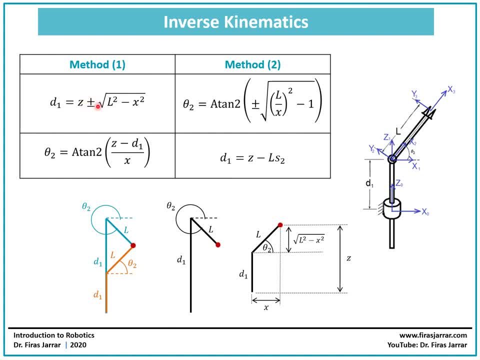 obtaining d1. we'll get two possible values for d1 and then we apply the formula for theta 2 to find the two values of theta 2 corresponding to each value of d1 in equation in method 2. we started by obtaining a value for theta 2 using this formula. 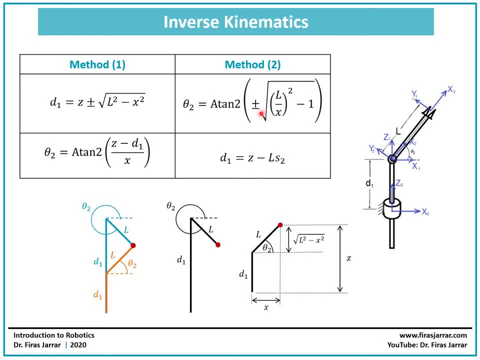 and turned out to be two possible solutions. then we substituted each solution into this formula to get the two corresponding values for d1. it's really interesting to see that the formulas don't really look this exactly the same, and this is totally okay and it's makes sense. 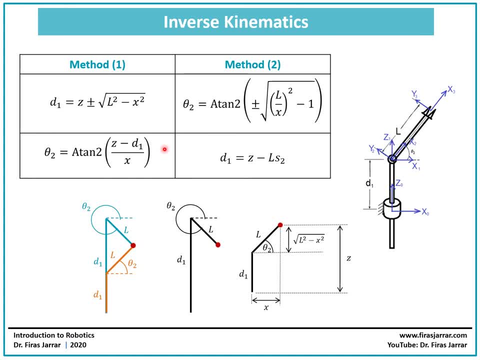 so it's not necessarily that we need to have the same expression to get the same value. it could be different expressions, but they will always talking about the same thing. so, for example, if you look here, d1 is equal to z plus minus under the square root, l squared by five into X, alpha, cosine, phi, equal to m z plus minus f, double minus y, sin awareness. 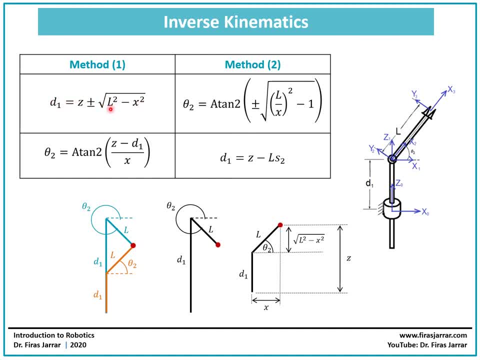 d1 is equal to z plus minus under the square root l squared byX time. let's use pointing here. I y divide my'd and keep the negative. 1 after that l squared minus x squared. l squared minus x squared, and the square root is in reality. 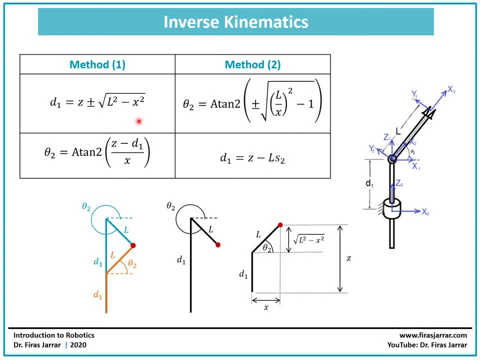 equal to l sine theta 2, so you can see both of them are really referring to the same thing. now, one way of to really, let's say, verify your solution is to try to think about the graphical approach. and so, for example, here we look at the method one we have it say, according to the 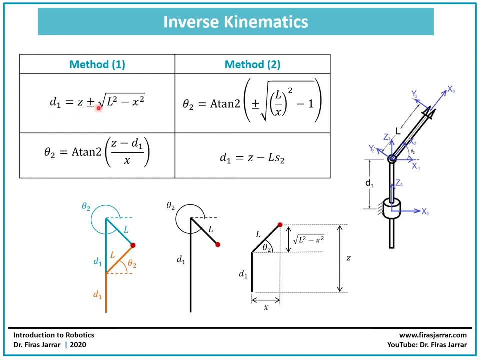 formula. it says that d1 is equal to z plus minus under the square root: l squared minus x squared. so let's look at it here. this is z, this is d1. what would be this small distance? here it's supposed to be: this is l and this is x. so l x minus l. 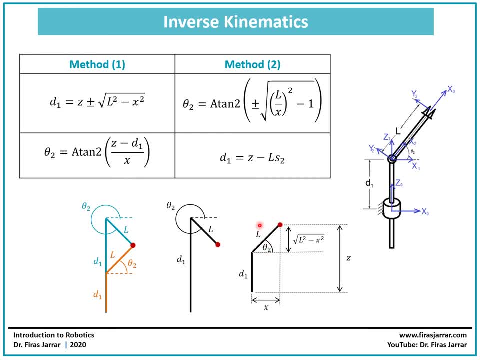 squared minus x, squared under the square root according to, for the girls, will give me this length here. so then i can relate z to d through what z minus this distance will give me this distance, which is this equation. and also, if you wish, you can also find theta 2 from: 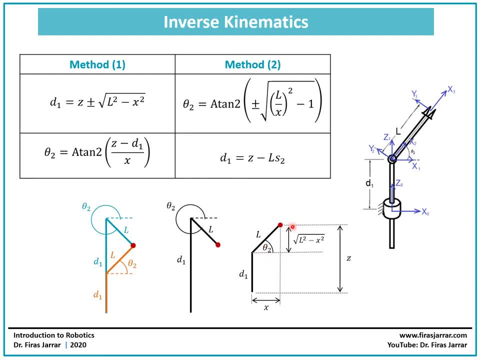 from graphical approach, tan theta 2 is going to be this distance, which is z minus d1, over this distance, which is x, from this right triangle. here it's always very useful- and i always recommend it- to try to relate the equations to the geometry of the problem itself and try to make sense of it sense. 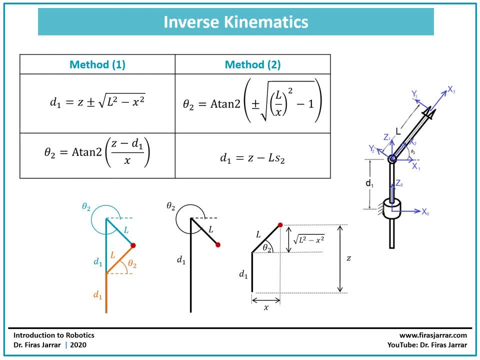 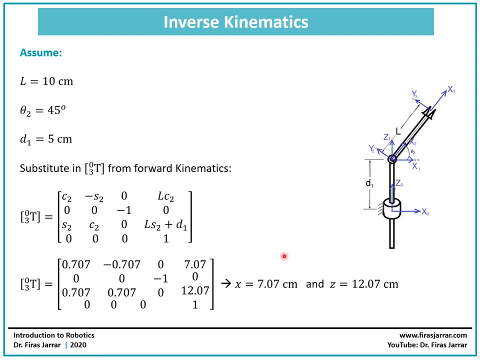 out of it. so, if you want, you can or make the doing, and when it happens that you can, always burning, with the help of those of the heat transfer, of the bullshit vacuum, you can make it. this נ now. another way to verify your solution is to assume numbers. 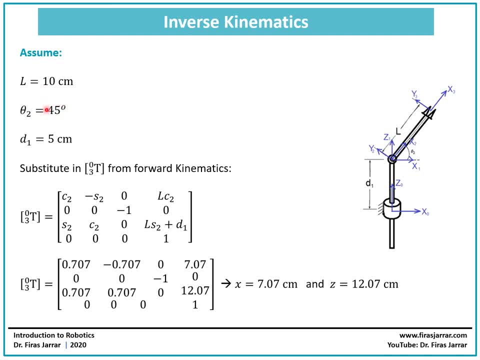 l. so we're assuming that l is going to be equal to 10 centimeters. if you want, you can assume 32 to be any angle. i'm assuming here that's going to be equal to 45´. also, d1 is going to be equal to 5 centimeters. you can choose any other. 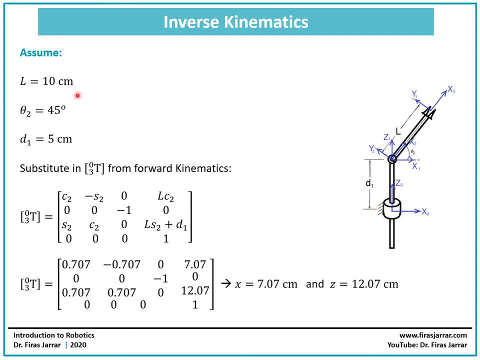 numbers, by the way, and then I'm going to substitute these into the result from the forward kinematics, which is the transformation matrix of 3 with respect to 0. so cosine theta 2 becomes cosine theta, and cosine 45, which is about point seven, or seven minus sine theta 2, becomes minus sine 45, which is minus. 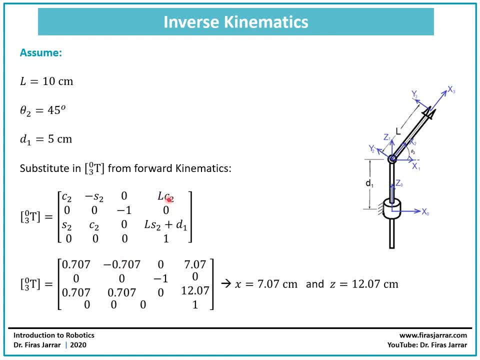 point seven or seven. L, which is 10 times cosine 45, is going to give me seven point or seven, and so on. the result of the fourth kinematics would be then X equal to seven or seven centimeters and Z equal to twelve point or seven. 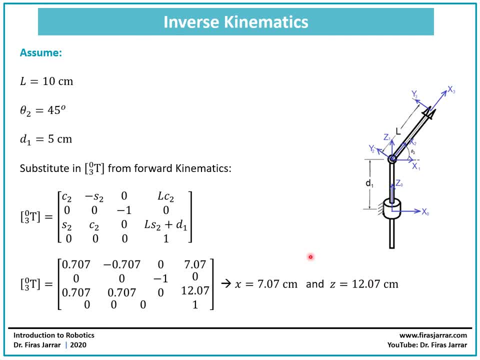 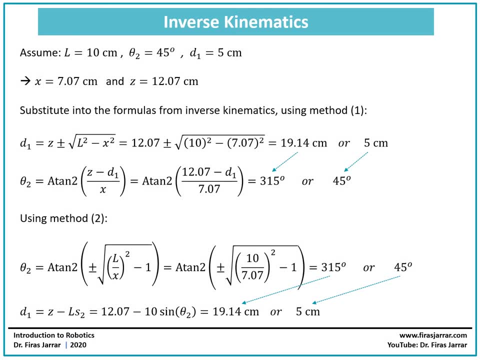 centimeters. can I take this result to the next slide again? I'm assuming the dimension here, which is that L is equal to 10 centimeters. I'm assuming that at a certain instance in time theta 2 could be equal to 45 degrees and d1 could be equal to 5 centimeters after. 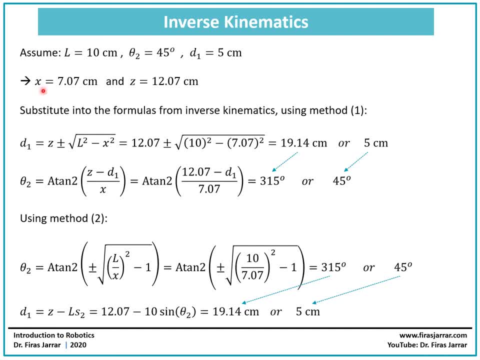 substituting these into the fourth kinematics, I got a value for X equal to seven point or seven centimeters and a value for Z equal to twelve point or seven centimeters. I will take these values and substitute them into the formulas obtained from inverse kinematics, using 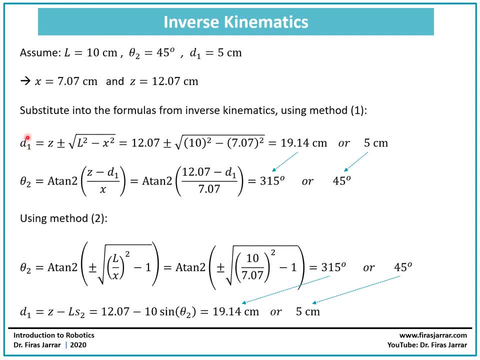 method one and using method two. from method one, I had a formula that gives me d1 equal to Z plus minus L squared minus X squared and the square root. so if you substitute for Z with twelve point or seven, for L with 10 centimeters and for X with seven or seven, as we have here, and since we 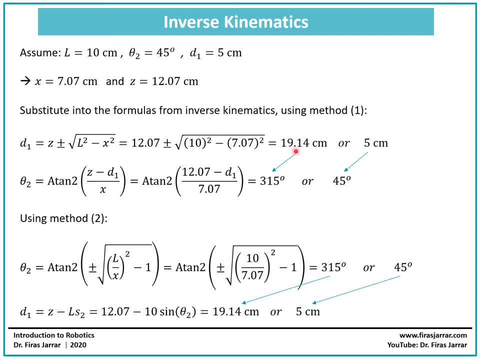 have plus or minus. this would give me two values, one values being nineteen point one four centimeters and one value being five centimeters. the same method we obtained a formula for theta 2 which depends on Z, d1 and X. so substitute for Z with twelve point or seven, for X with seven point or seven. 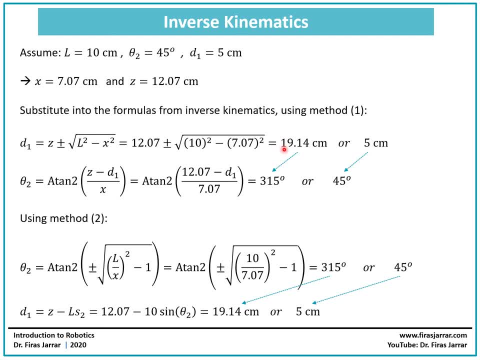 and then for d1, we're going to substitute once with nineteen point one, four and once with five centimeters. when we substitute it for D with a nineteen point one, four centimeters, this gave us an angle of minus 45 or 315 degrees. when we substitute it for d1 with five centimeters, this gave us an angle of 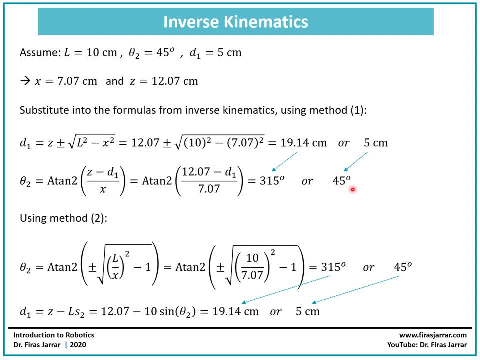 45 degrees. so what we got here is that d1 could be five centimeters and with a value for theta 2 of 45, and notice that these are the same values we started with. we have started assuming a value for d1 to be five centimeters and theta 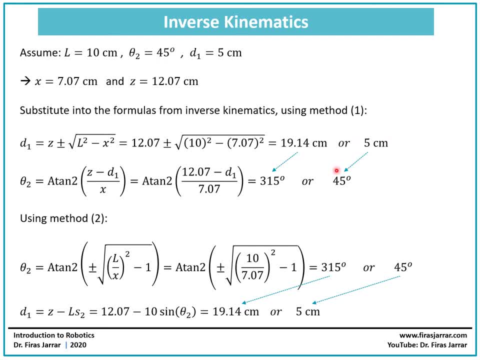 2 to be 45 degrees and this validates our approach. so if you started with a certain assumption for the joint variables, you went through the four kinematics, you found the corresponding position and then you took the position and substituted that into the inverse kinematics and you got the same joint variables that you started with this in. 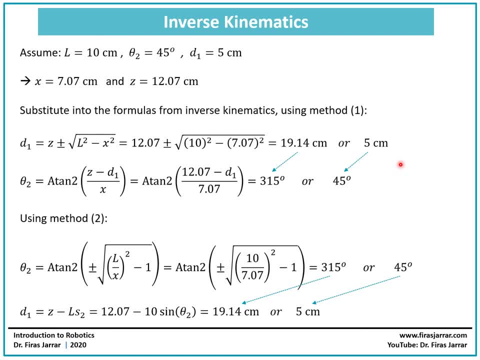 somehow also verifies on or validates your approach. In addition, you will see that we'll get a second solution, because we agreed that for this problem we have two possible solutions. Now let's look at method 2, because some of you may not be convinced that. 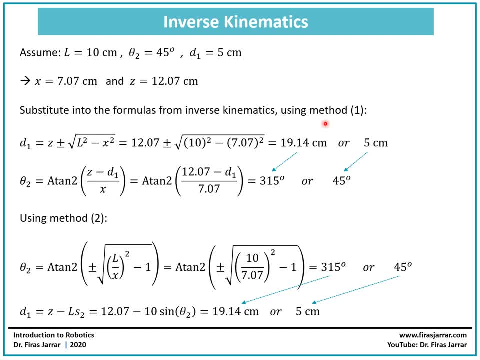 both methods are correct or both methods will give me the same answer. So let's see. We start with theta 2.. Theta 2, according to method 2, is equal to a tan 2, which is tan inverse of plus minus l over x squared minus 1.. l is 10 centimeters and x was found to be 7.07.. 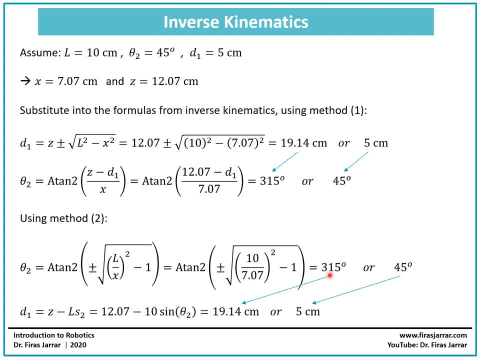 This would give me two answers: either 315 degrees or 45 degrees. Now, d1 is equal to z minus l, sine theta 2.. z being 12.07.. l is 10 centimeters and sine theta 2, sine of either 0.. 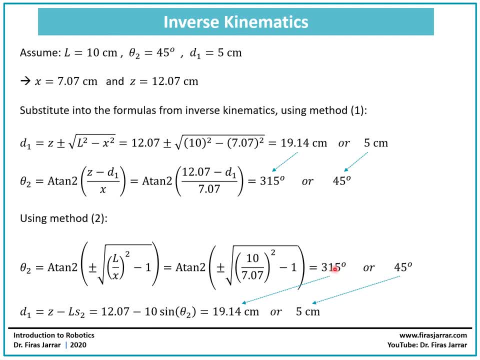 315 or 45. So if you substitute 315 here for theta 2, this will give you 19.14 centimeters. If you substitute 45 degrees, this is going to give me 5 centimeters. So I'm again getting the. 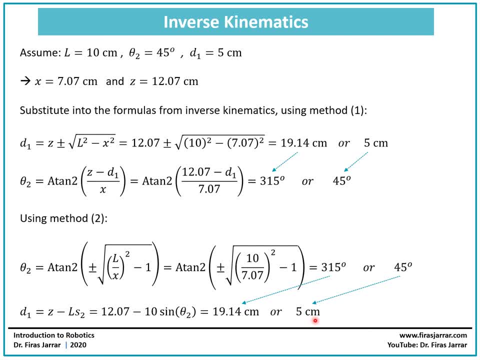 same two pairs. If d2 is 5 centimeters, I will have an angle of theta 2 of 45 degrees to reach the same end effector position. If I had a value for the d2 being 19.14,, this corresponds also to an angle of theta 2 equal.